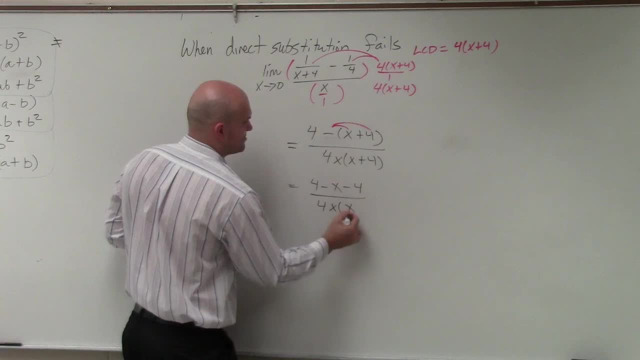 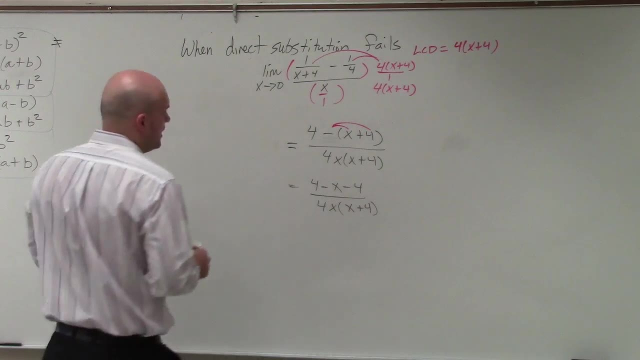 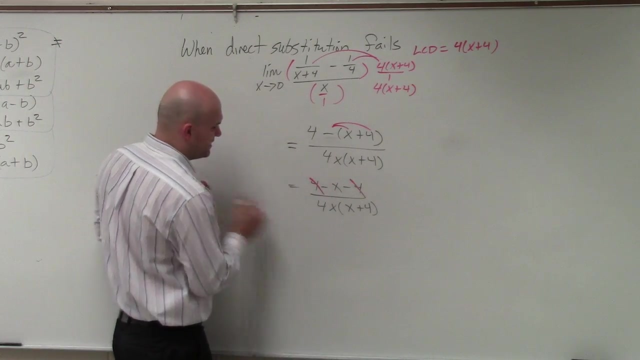 Divided by 4 times x times x plus 4.. Again you could distribute, but let's just leave that distributing out for a second. What we notice here is the 4 and the negative 4 divide out. So therefore that's just going to leave me with a negative x. 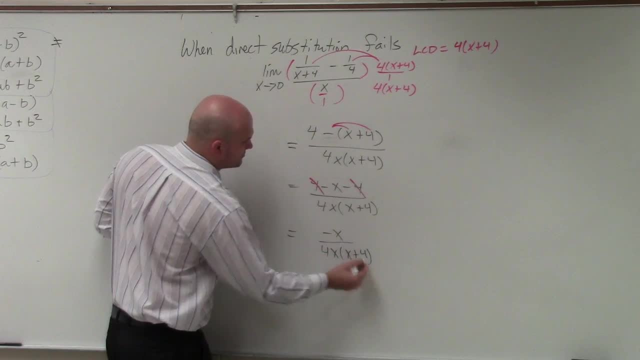 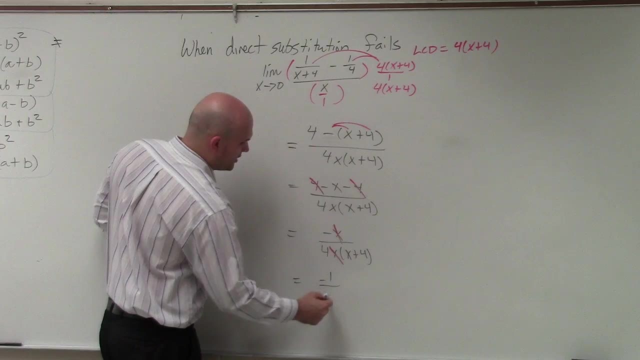 over 4x times x plus 4.. Now my x's divide out, So it's leaving me with a negative 1. So that leaves me with a negative 1. So that leaves me with a negative 1. So that leaves me with a negative 1 over 4 times x plus 4.. 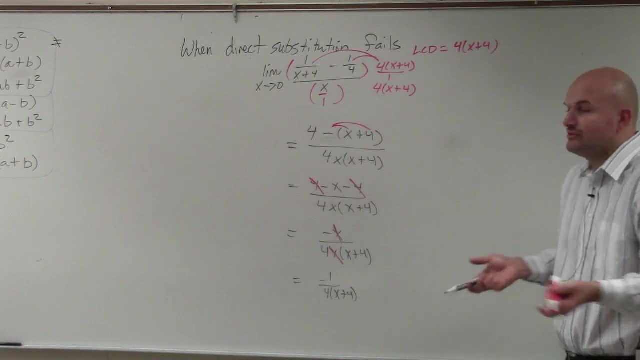 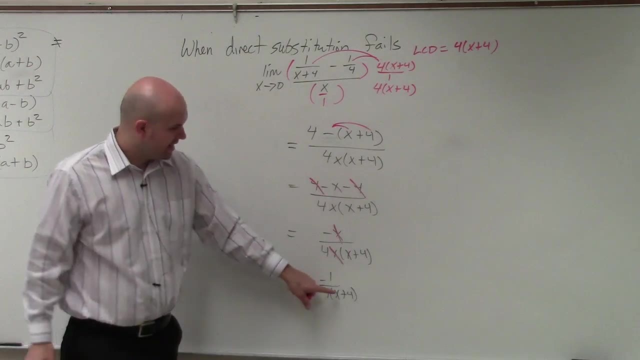 And again you can distribute it. but we don't really need to. All we're doing is going to be evaluating for 0. And when I plug in my 0, I get 0 plus 4 is 4.. 4 times 4 is 16.. 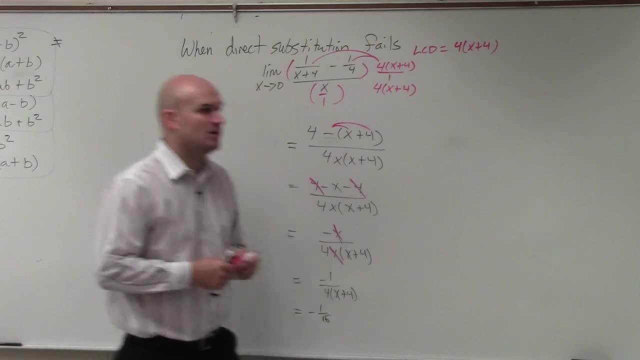 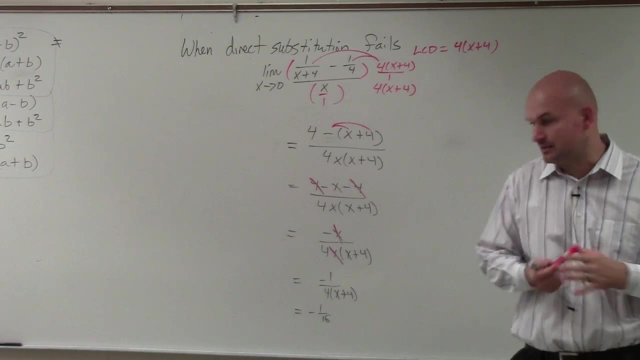 So my final answer is negative: 1, 16th. So yes, I could factor it, I could distribute and simplify it, But I don't really need to because I'm just going to be direct substitution. that back in. Does everybody see that? Yes, OK. 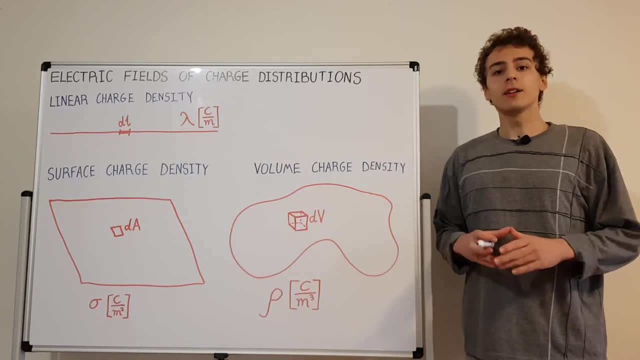 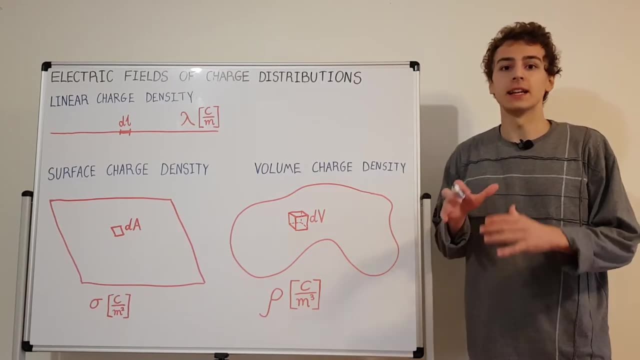 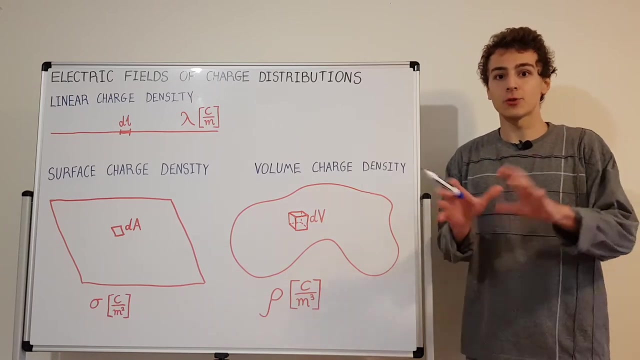 In this video I'm going to talk about charge distributions and how they can produce electric fields. We're going to have a look at some of the concepts in calculus and integration that you can use to solve these types of problems. So what is the area of electromagnetism that these types of 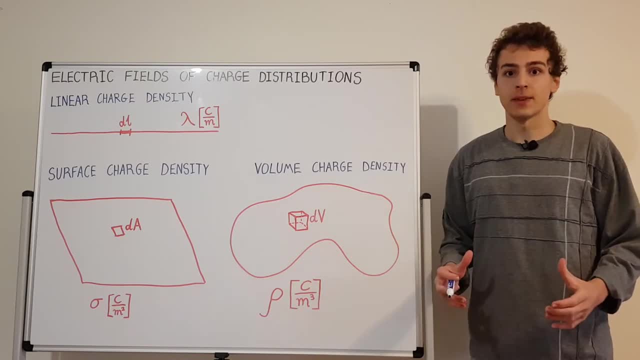 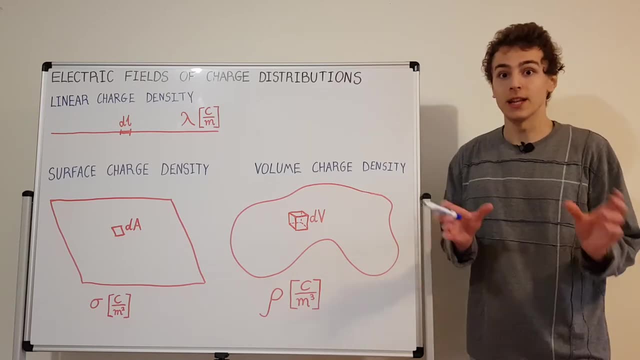 problems emerge in. Well, it's electrostatics, And statics means that things don't change with respect to time, And electro that's the prefix for electric fields. So electrostatics are when you don't have changing electric fields, you just have charges that have always been there, and 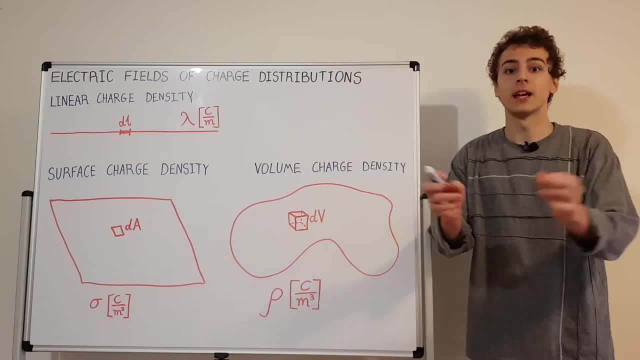 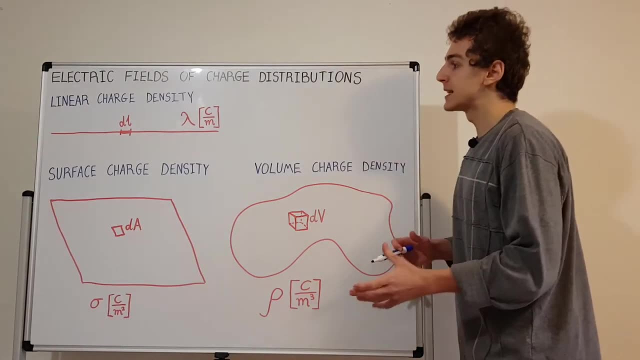 they're not going to move. So there's always a consistent electric field emanating from these charges. Let's have a look at some common charge distributions. So a lot of the time you're going to see a line of charge like a wire that's charged but there's no flow. Remember this is electrostatics.